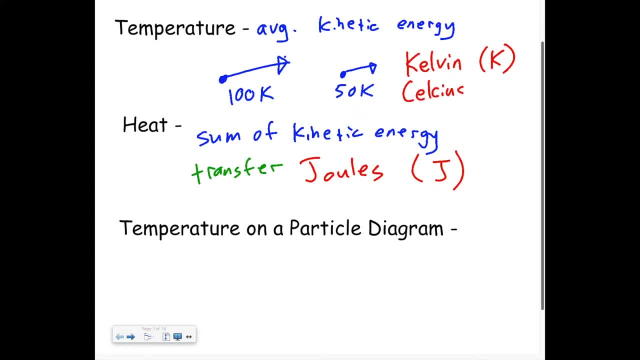 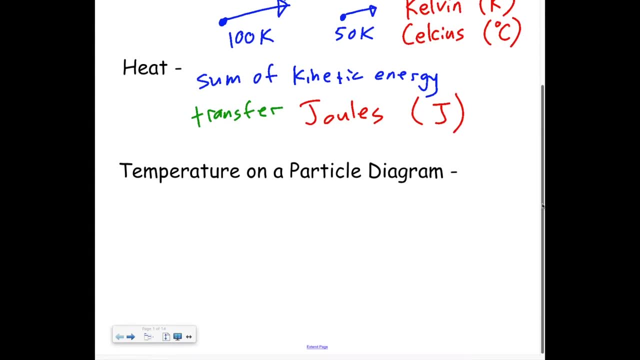 So it's going to be K or Celsius, and that's written in degrees C, which you've probably seen before. Now let's show this on a particle diagram. I kind of drew it a little bit before, but if we were to draw two different things, 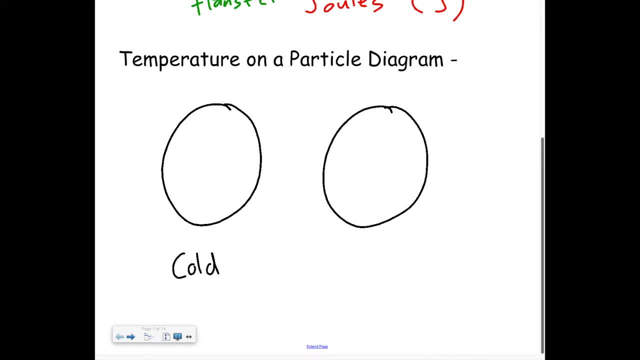 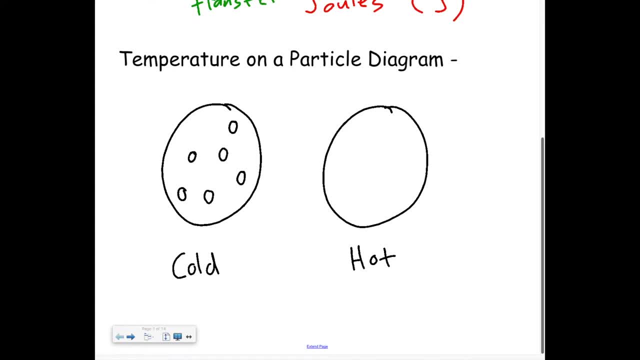 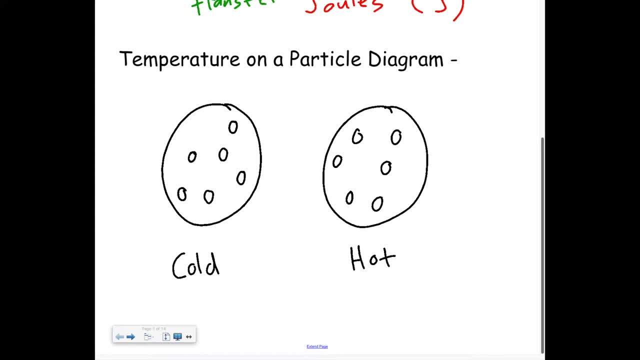 The only difference is their temperatures. So to really show a temperature, you have to show the arrows, You have to show its direction. So when we show arrows- there's two- it tells us two things: It tells us the direction and also the length of the arrow shows the speed of the arrow. 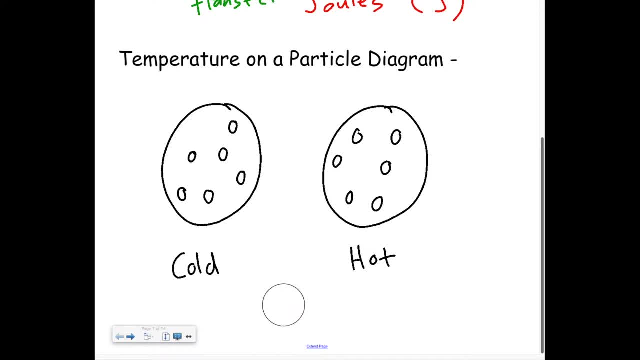 So we have to show the speed of the arrow. So when we show arrows- there's two- it tells us two things. So the direction and the magnitude of the arrow is what's important. So here we go. So a cold one. I'll do them in different colors, why not? 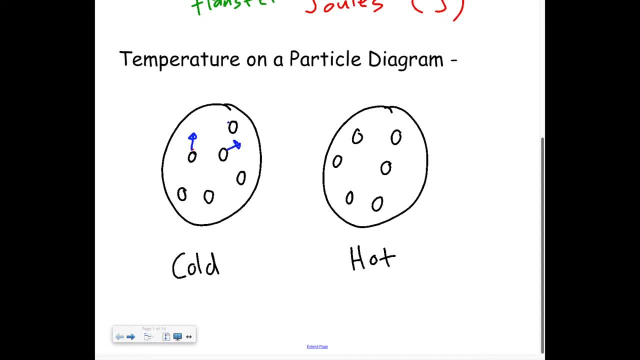 So cold one is going to have these shorter arrows and they're going to be moving around it different. They're not all be going the same way, they're just kind of randomly moving. But they all have relatively short amounts of arrows. They don't all have to be the same length, just kind of relatively short. 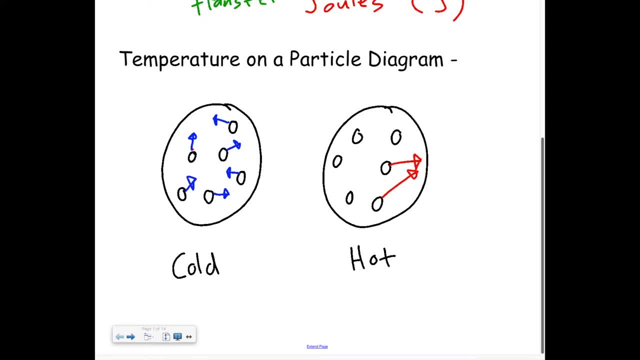 And now the hot ones will have longer arrows. Some of them are a little bit longer than others, but that's okay. And again, they're moving in random motions. I just picked a direction and drew them And you would just need to make sure to distinguish between shorter and longer arrows. 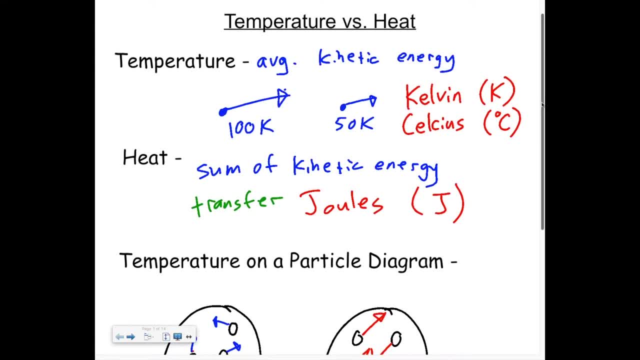 Alright, so I hope that sums it up. Temperature is measured in Celsius and it represents the jiggliness of the molecules, Right? So this is representing the motion of the molecules, And then the heat is actually representing a transfer of energy. okay, 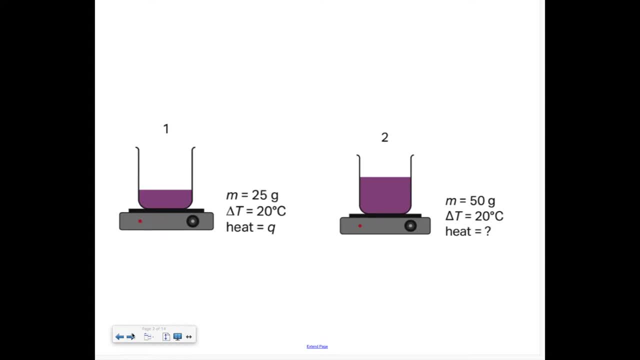 So let's move on and let's think about the heats of two different objects. okay, So we have number one and number two. So for number one, it has a mass of 25 grams Delta T of 20 degrees Celsius. 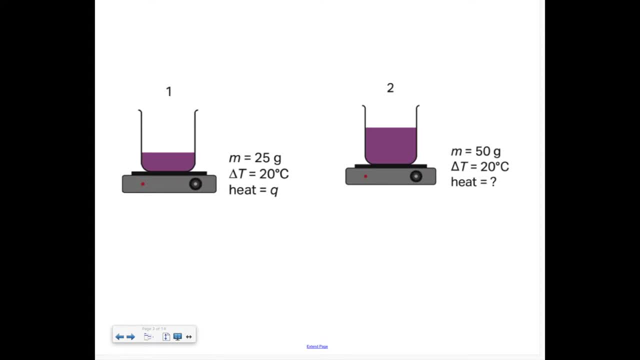 Its heat is represented as the letter Q. So for number two, its mass is 50 grams, but its temperature, its delta T or its change in temperature, is 20 degrees Celsius. Still the same, So the same temperature, but now it has double the mass. 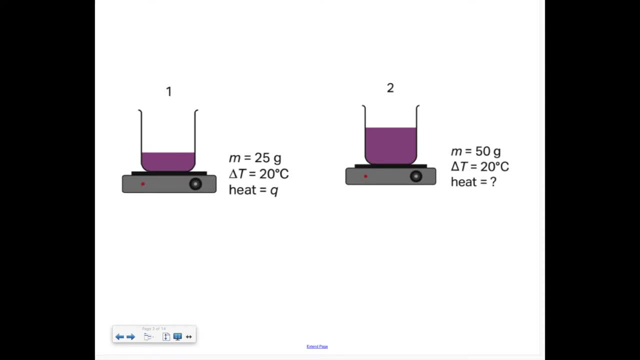 How much heat is it going to require to heat up this substance to the same temperature? So you might be able to understand that if, since there's twice as much stuff To get it to the same temperature, right To get it to the same temperature, you're going to need twice as much heat. 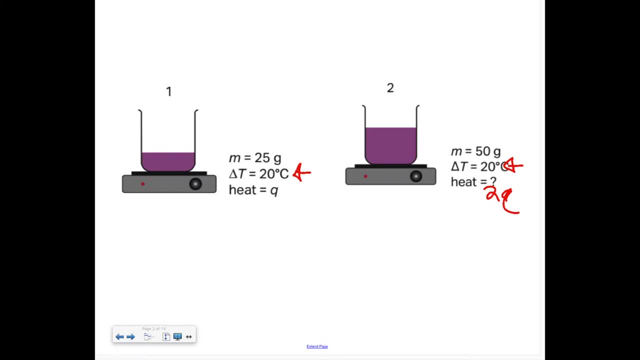 So you would need two Q. So as the mass increases, then it's proportional to the heat. Heat is written as the letter Q. Now for the next one. all of mine are a little too low. For the next one. For number one and number three, the mass is 25 grams. 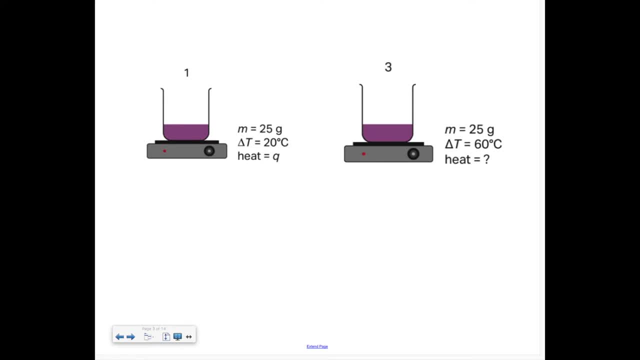 And to get it to the temperature of 20, an increase, a temperature of 20 degrees Celsius. And then for number three you have: the mass is still 25 grams, but you want to increase the temperature by 60 degrees Celsius. 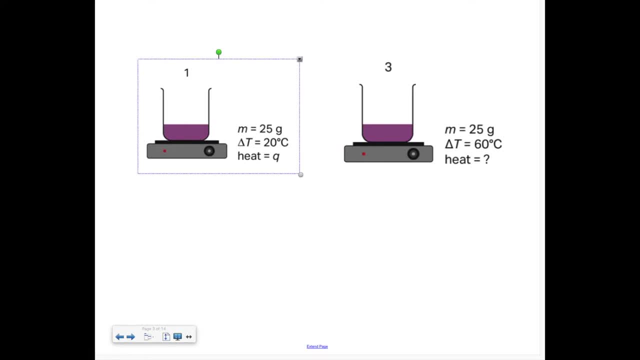 So it you get. you want to increase the temperature by three times the amount. Okay, So how much heat Would you need If the mass stayed the same? right, So, hopefully, pause and think about that And you probably, hopefully maybe- came up with you would need three Q as well. 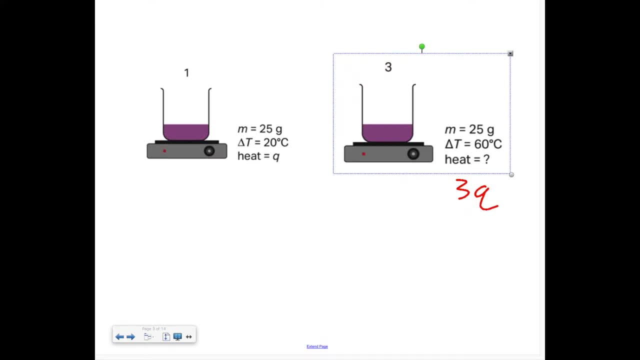 So if you, if you have the same amount of mass and you want to increase the temperature by a certain proportion, then also the Delta T, or the change in temperature, is also proportional to the heat As well. So as the heat, as the temperature goes up, the heat will go up. 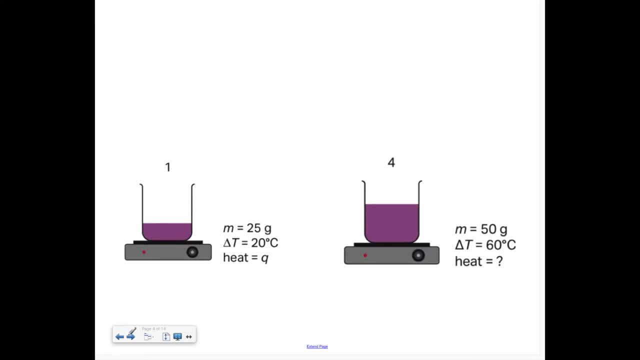 And then the last one. let's see if we can flex our brains. I want you to pause the video and take a look at this one. So what do you think is going to be the heat? We've now changed the mass, So we've doubled the mass and we've also tripled the temperature. 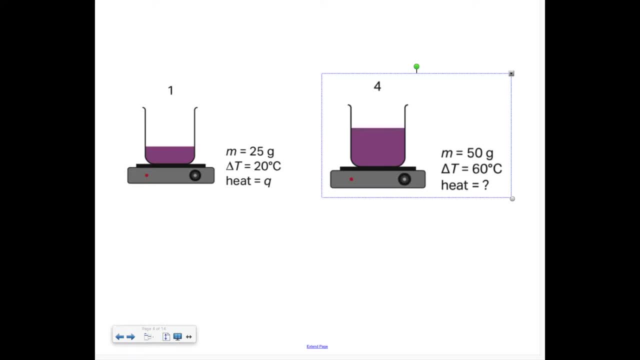 So what's going to be the heat? So it should be 22.5.. 2Q times 3Q, right, which would actually end up being 6Q, not 6Q squared. it should be 6Q. okay, should be 6Q, so 6 times the original heat. 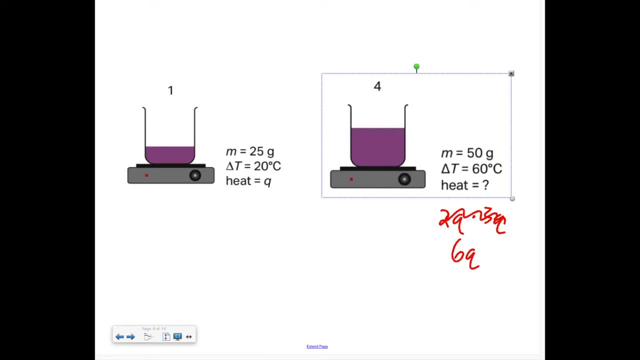 I hope that made sense and what the idea was. just to understand that heat depends on the mass and it also depends on the temperature. And there's one other thing that it does depend on, and we'll just skip ahead- and it depends on something called the specific heat, which is, like this, proportionality constant, and we'll explain more about that in a second. 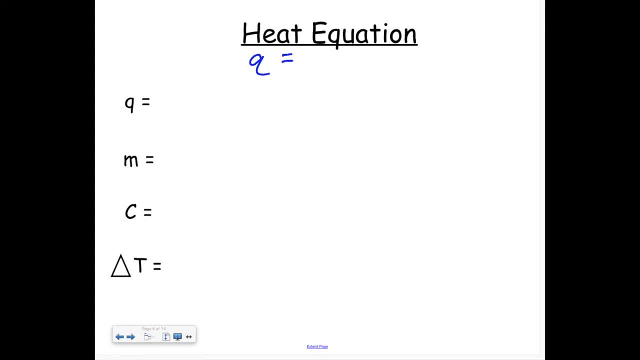 So the heat is equal to the mass times, the specific heat which has the letter C and times the delta T. So this is all in your notes: Mass times C times delta T. So delta delta means change. so whenever I say delta T I mean change in temperature. 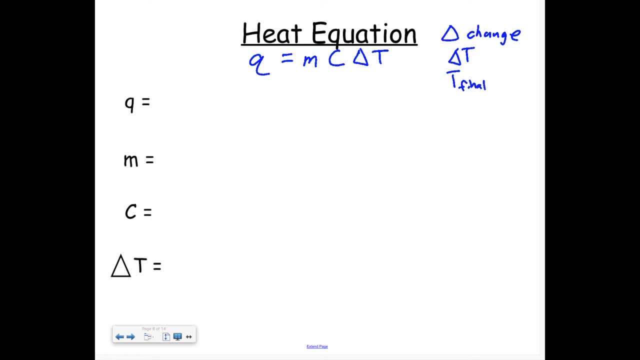 So that is written as T final minus T initial. Okay, so Q is going to be your heat, and that's written in joules. M is your mass and that's written in grams C is your specific heat- almost about ready to talk about this in a second- and that unit is joules per grams degrees Celsius. 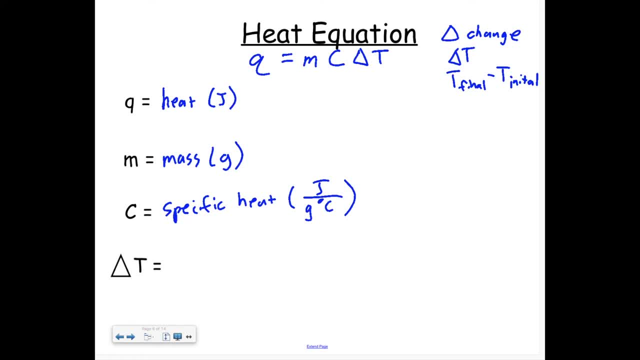 And then temperature or delta. T is your temperature, your change in temperature, and that is your T final minus T, initial. okay, And its unit is either degrees Celsius, All right, so that's specific heat. Well, if you think about it, a piece of metal is going to heat up differently like a piece of iron, like your iron frying pan is going to heat up differently than water, correct? 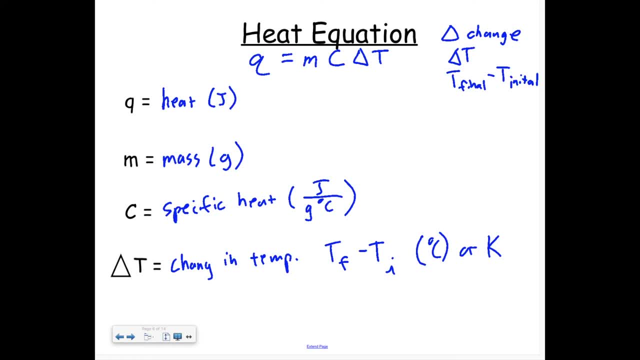 Iron gets hot a lot faster and it cools down a lot faster than water. does You know? water can stay hot for quite a long time. Okay, So it depends on the substance itself that dictates what the specific heat is. So this is an intensive property. 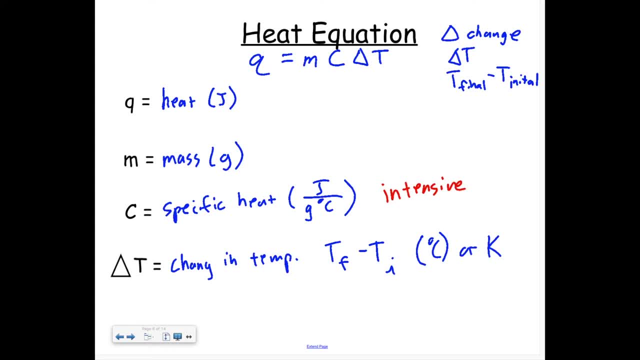 This is a value that changes per substance and every substance is unique and it never changes for the substance. It does not depend on the mass, It doesn't depend on the amount, But it does depend on what the substance is. So our lab today is going to be to find the specific heat of a certain metal, and it's going to be great. 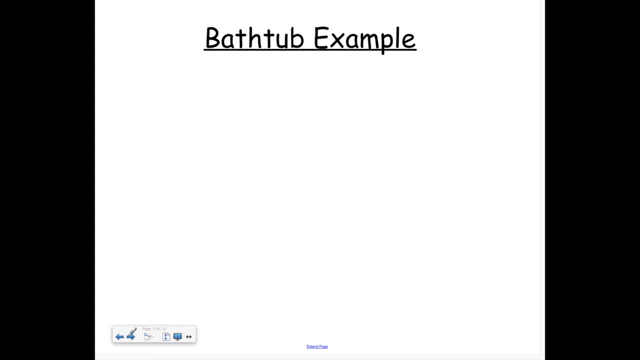 So one last thing, one extra thing before we get into the lab, I want you to think about a bathtub, right? So? and you're filling up your bathtub here, and you start filling it up, and you have lots and lots of hot water. 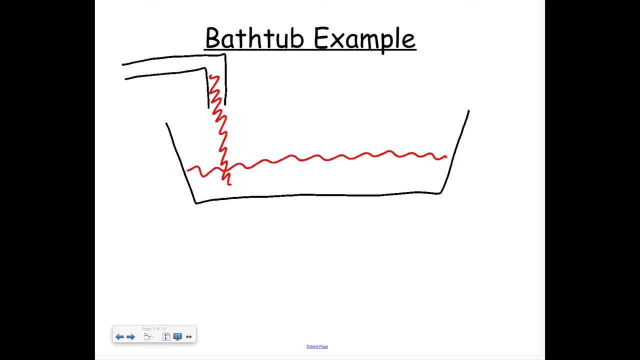 And you end up filling- You're filling it up too much with hot water- And then, whew, you start to get in and you're like, wow, wow, wow, that's way too hot. So what do you do? 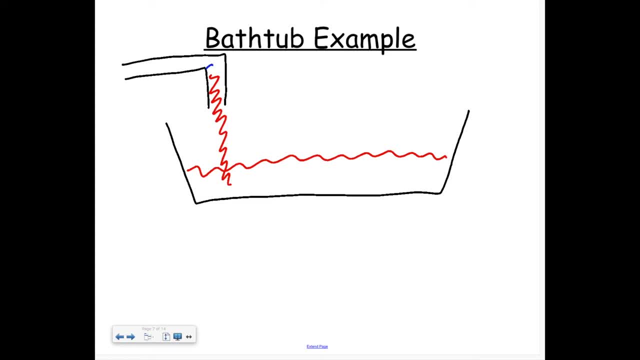 Well, you turn the hot water off, right, And you start trying to mix in a little bit of cold water, right? So what happens with that cold water? It lands in there Now. does it instantly change the temperature of the whole thing? 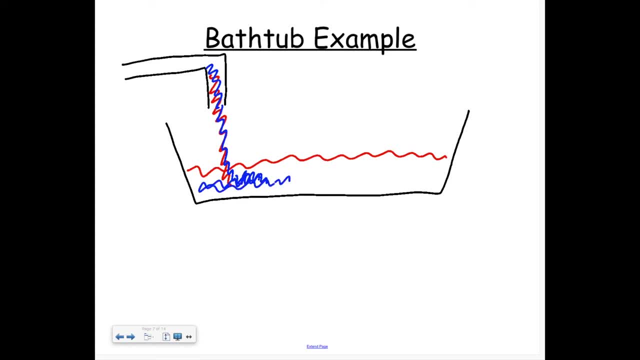 No, because this side is more cool than the other side, right, But eventually it will also. It will all kind of settle out and all of that: the hot water and the cold water will mix and will mix all together, right. 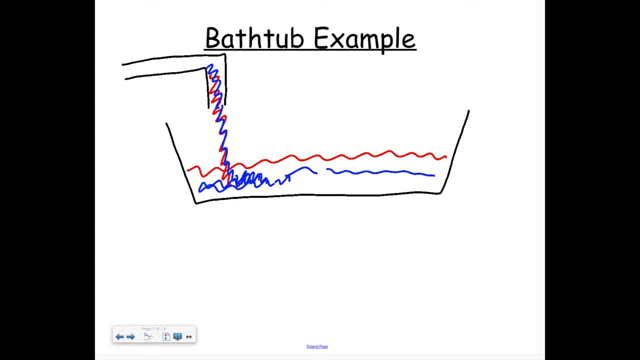 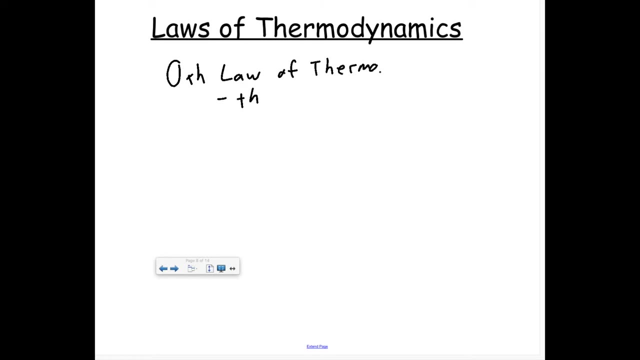 And you kind of understand that how the temperatures will eventually equilibrate. So that's the same type of thing that we're doing, And what that's called is that's called the zeroth law of thermodynamics, And that's essentially telling us that there is some type of thermal equilibrium. 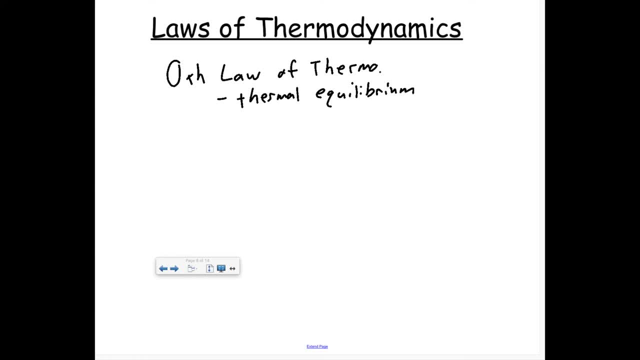 But that is just like the bathtub example: If you mix in hot water and cold water, they will eventually come together. So now the other one that we need to make sure we understand is the first law, the first law of thermodynamics, And that says that energy cannot be created or destroyed. 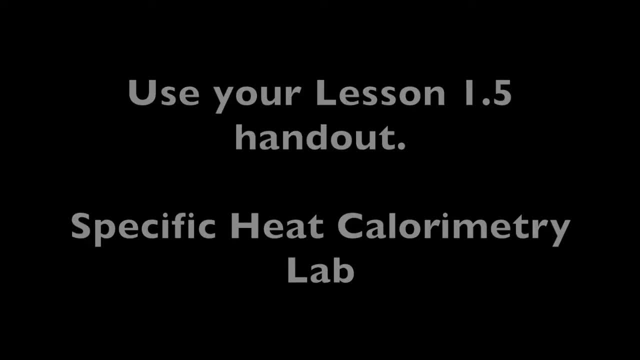 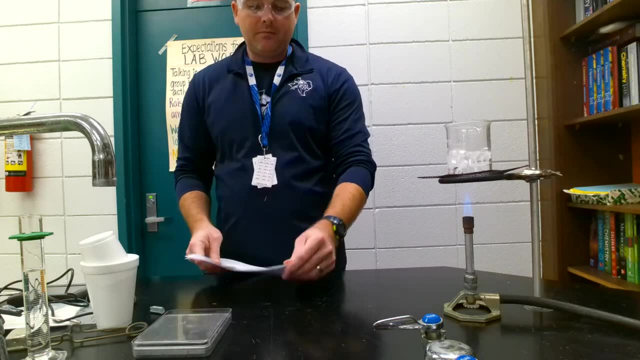 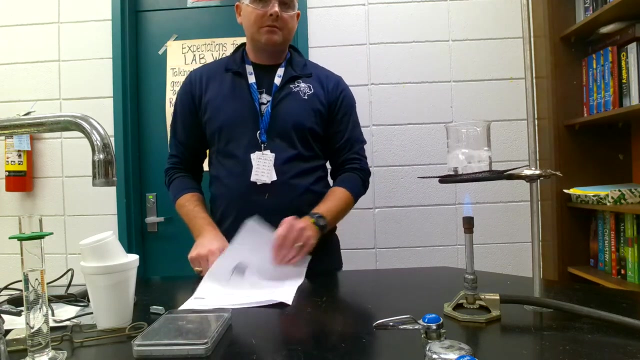 I hope that helps. Okay, so here we go. So we are going to collect our data for our calorimetry experiment. You have- You've kind of already understood exactly what the Q equals MCAT formula is. So what we're going to do is we're going to perform a very simple experiment that involves heat transfer. 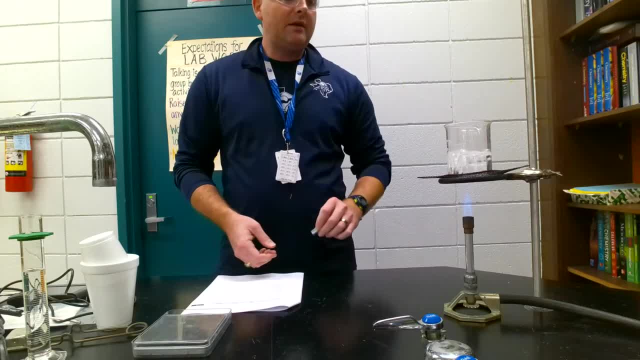 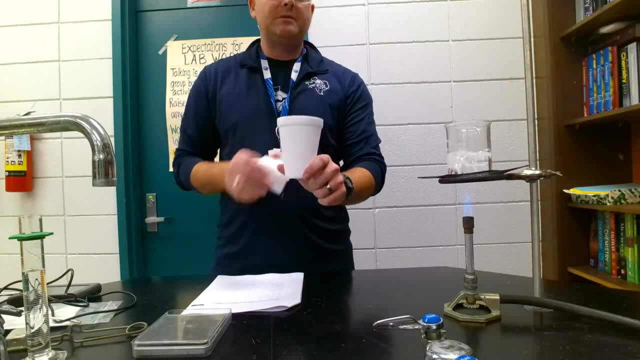 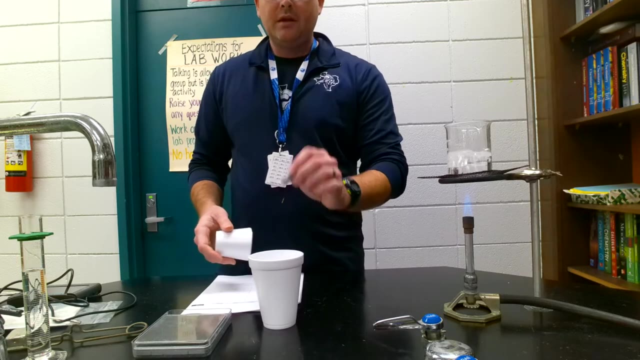 We're going to heat up this piece of metal in this water- hopefully before the water goes away- And then some cold, cool, room temperature water is going to be in here. We're going to transfer that piece of metal into here And then we're going to record how much. 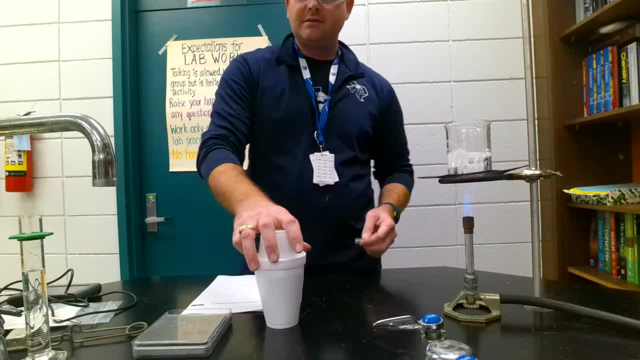 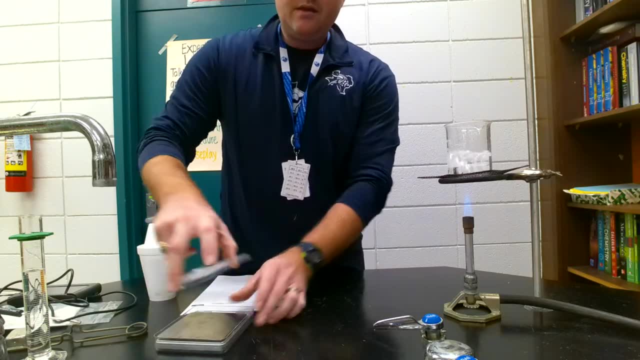 How much the water temperature changes. Okay, so that's essentially the gist of the thing. So the first part is to find the mass of the metal. That's going to be important. Remember that M in the MCAT equation stands for mass. 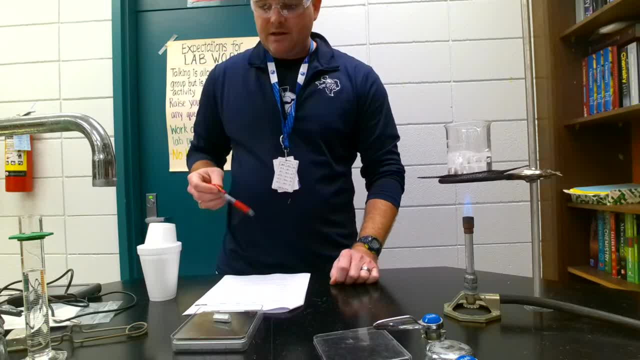 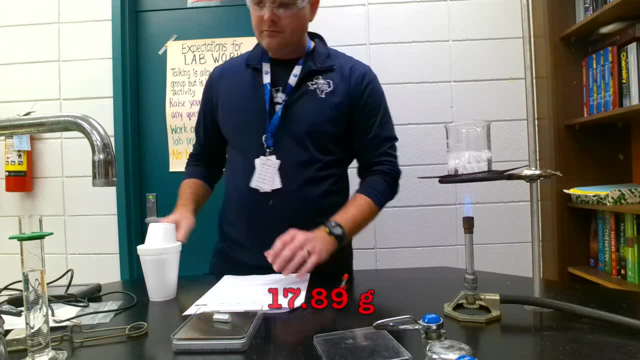 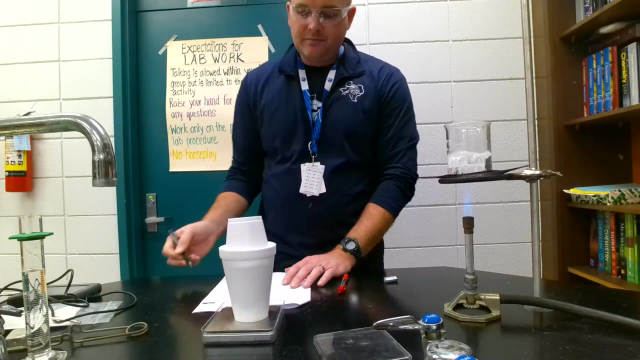 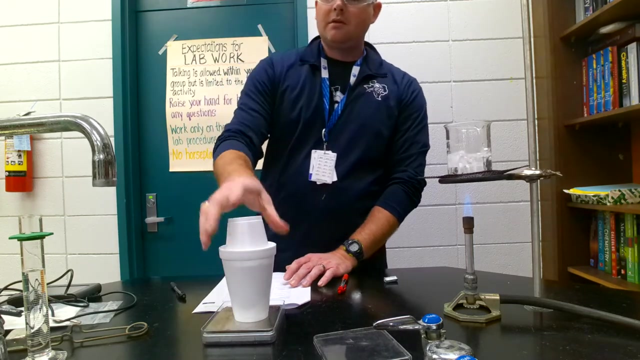 So And the mass is 17.89.. 17.89 grams. Then we'll find the mass of the calorimetry, And that's this styrofoam cup thing And that is 5.45 grams. And then we find the mass of the calorimetry and the room temperature water. 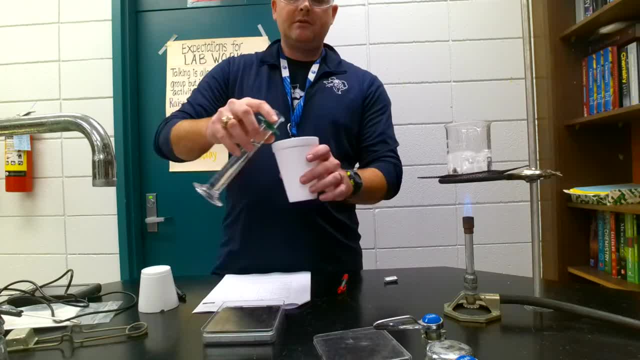 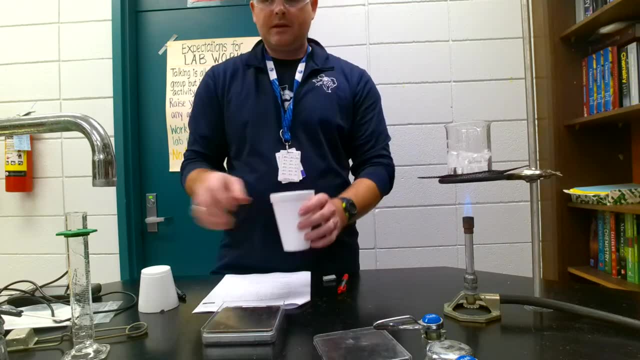 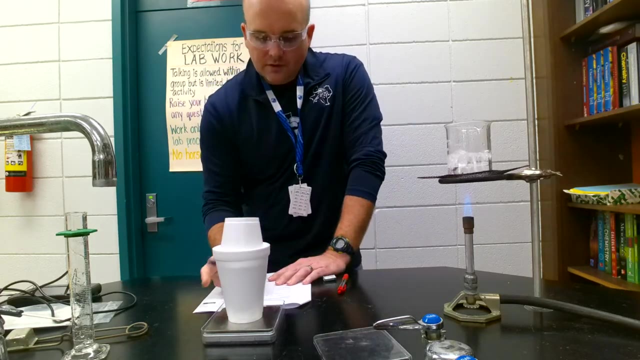 I don't mean this water, I mean room temperature water. Okay, Now, this is enough water to cover our sample, our metal, Just a little bit. I know you can't see it, So we're going to find That, And that is going to be 46.94 grams. 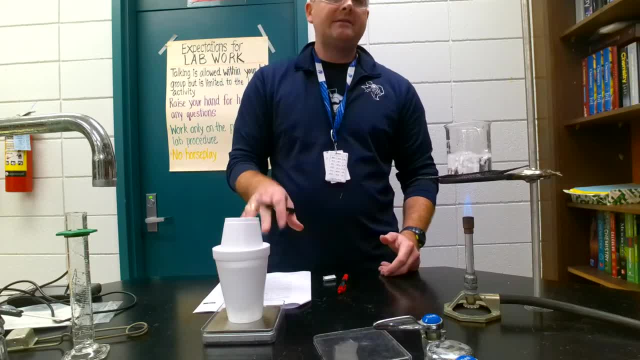 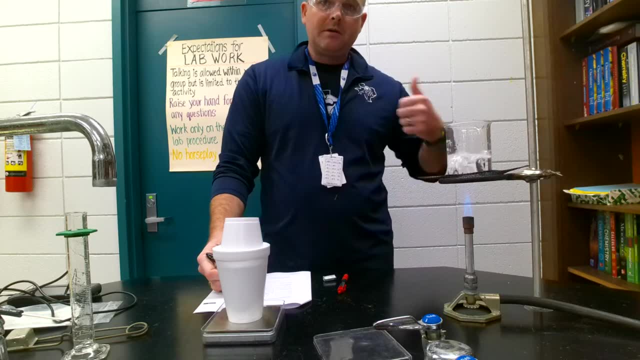 Now I don't necessarily care the mass of the calorimeter, I really only care about the mass of only the water. So you take the mass of the calorimeter plus the water, subtract it by the mass of the calorimeter and you have the mass of the water. 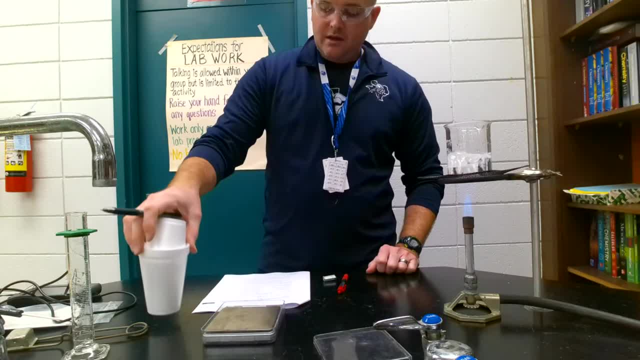 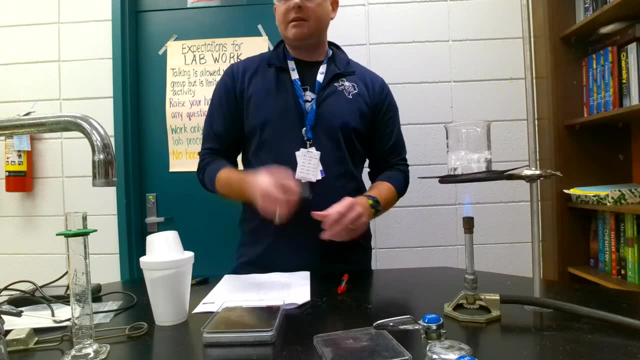 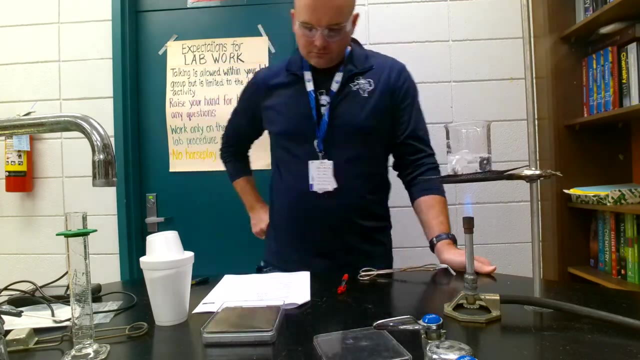 So that is the next blank. You can do that one yourself, So. So Then we're going to take the metal and I'm going to place it into there and let it heat up. Okay, So the metal is heating up right now. 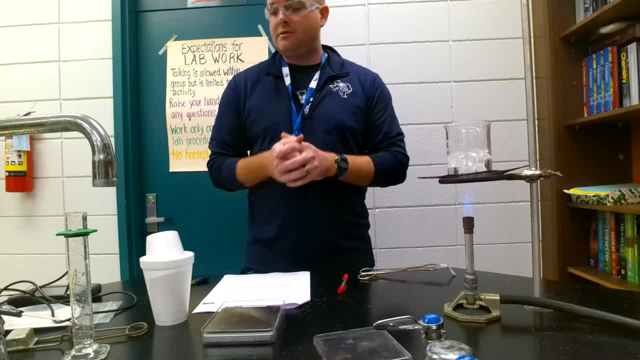 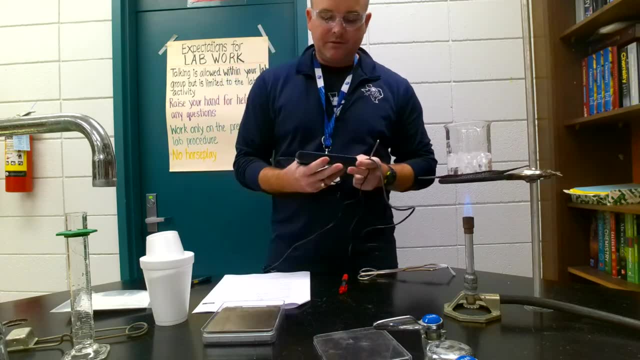 And eventually it will get to a, It will get to the temperature of the boiling water. Okay, So just to prove to you how, When does water boil, At what temperature? Right, It should be 100 degrees Celsius, right? 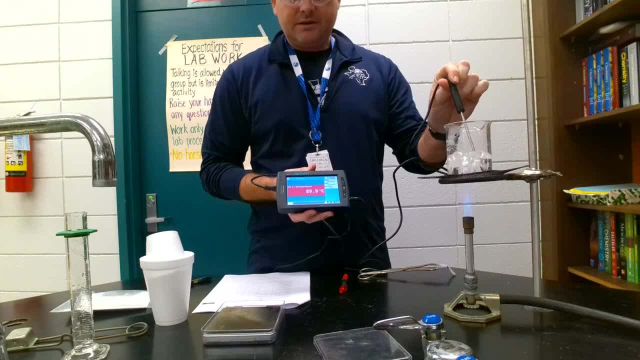 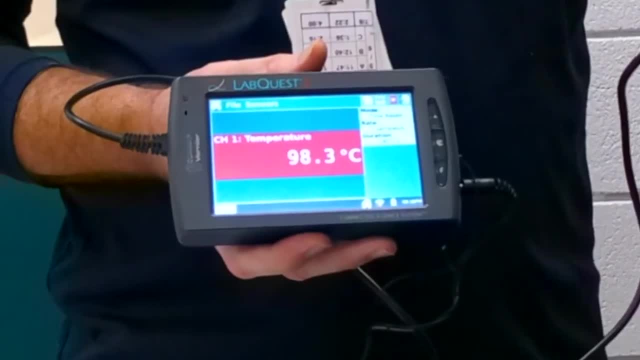 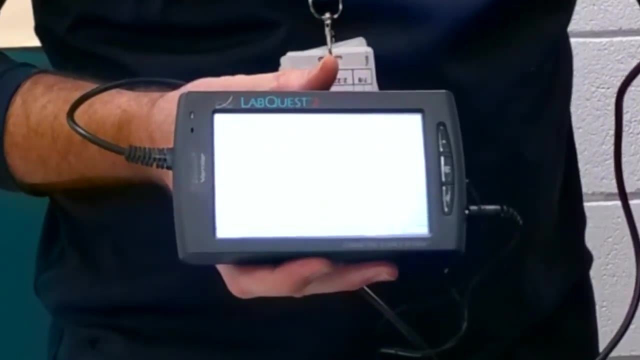 So If we put that in there, you can see it: climb, climb, climb, climb, And it should get right up to 100.. My finger is getting hot. Yeah, So it will get right up to 100, but it won't. 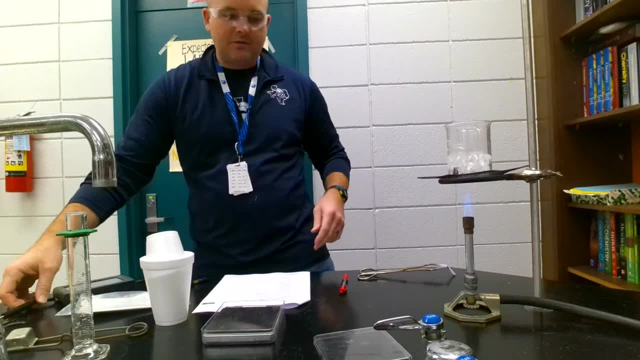 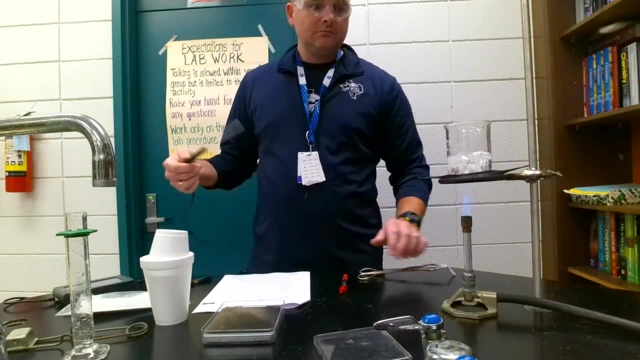 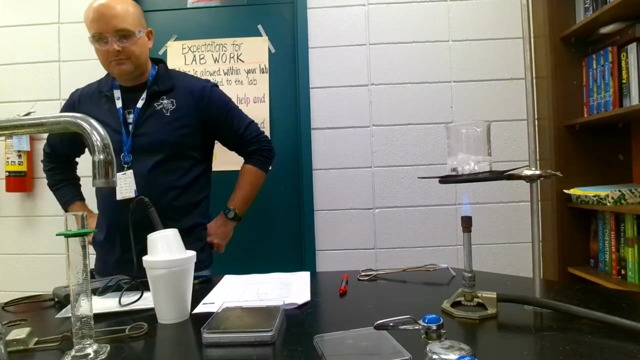 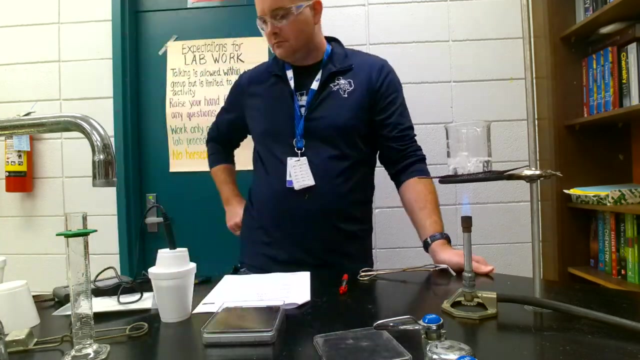 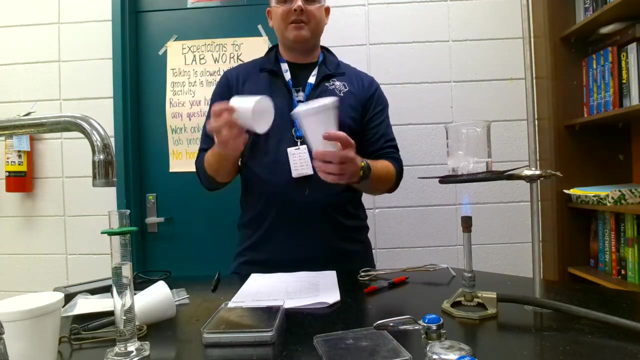 It won't go any farther. My finger is getting hot so I pulled it out a little early And I want to make sure this has time to cool down. Okay, So we had a. Um, We had a valuable flaw in our experiment. 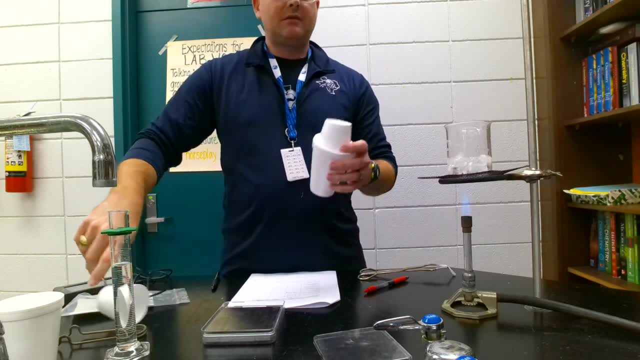 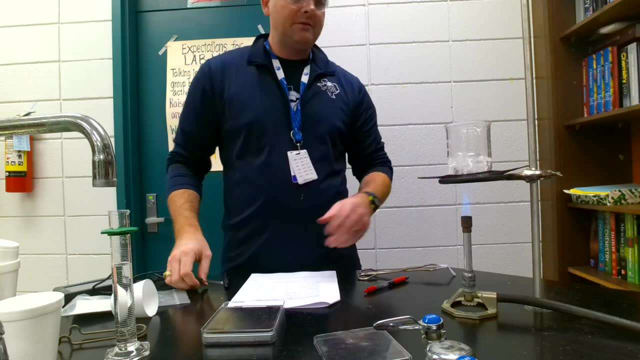 What was happening was that this calorimeter was too tall so that the thermometer wasn't actually touching the water whenever I put it in. Normally, I use more water because we use more sample, So I went and got a new one. Okay, This is going to change our data. 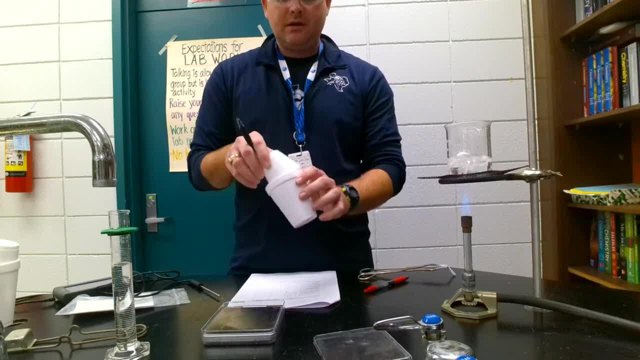 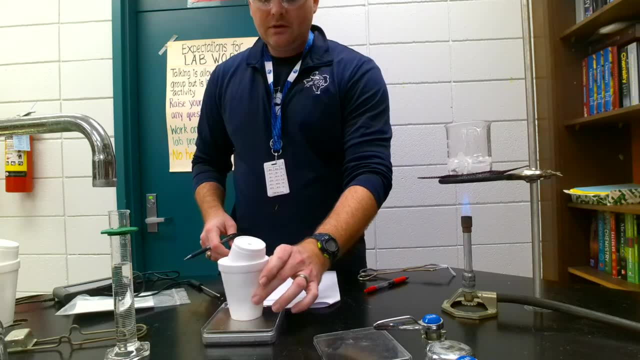 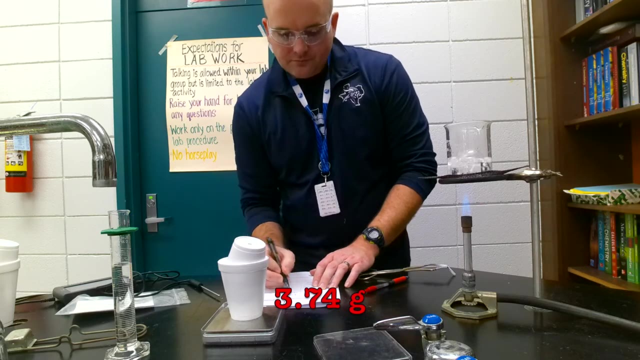 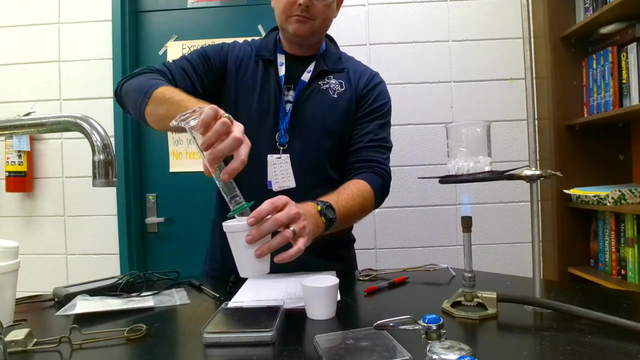 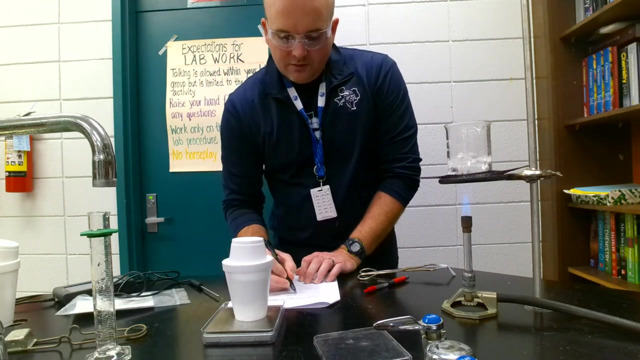 Okay, So the mass of the calorimeter, the new mass of the calorimeter- this is the one you should write down- This is 3.74 grams, And then the new mass of the calorimeter and the water is 45.17 grams. 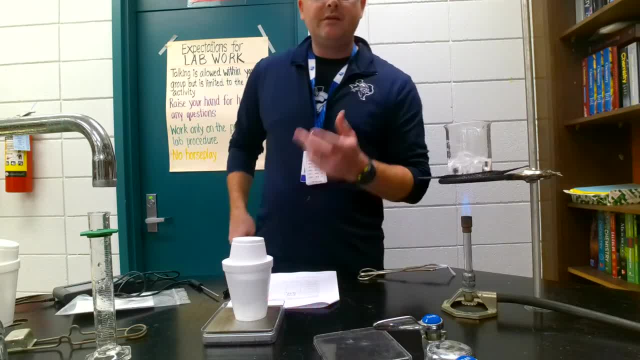 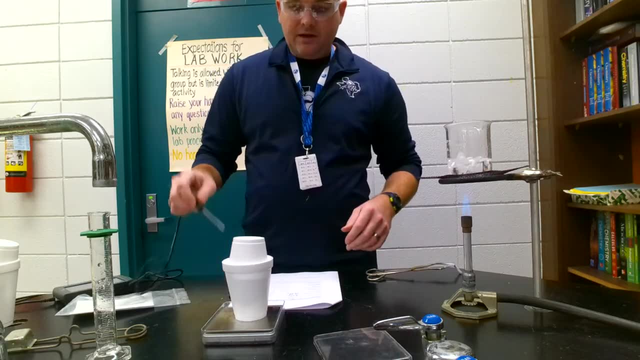 It doesn't exactly matter how much water I have, I just need to have enough to cover the metal and also touch the thermometer Um, And I just record that mass. So by now you should be able to calculate the new mass of water. 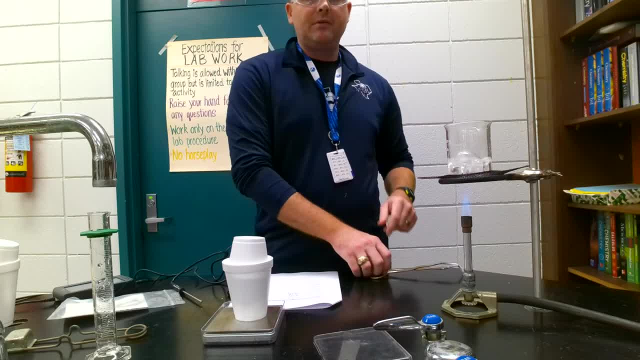 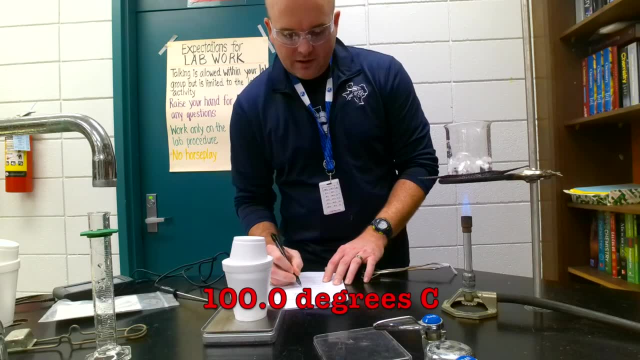 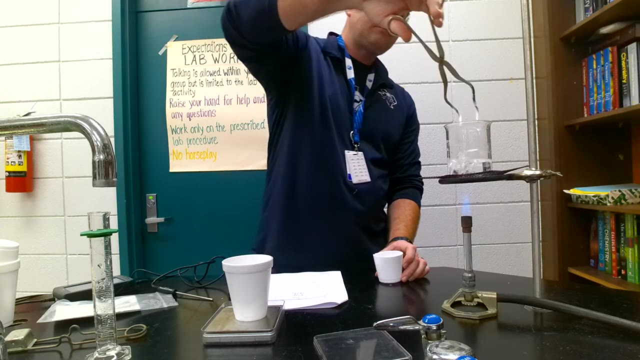 And now the initial temperature of the hot metal sample should be 100 degrees Celsius- 100.0.. So please write that down: 100.0 degrees Celsius. And then we are now going to take this and we're going to measure the initial temperature of the calorimeter. 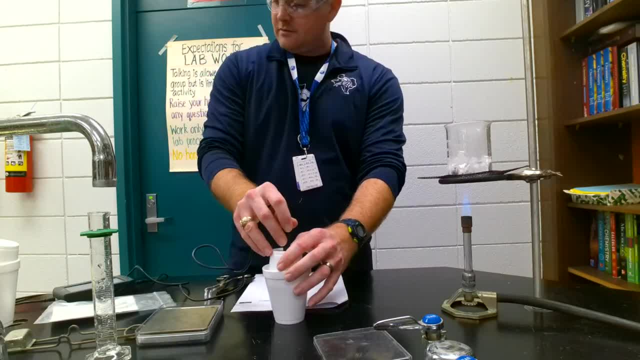 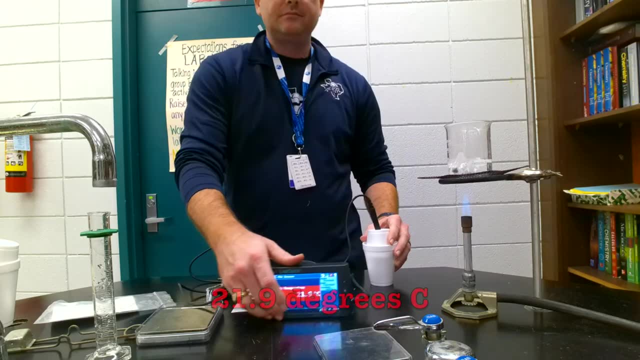 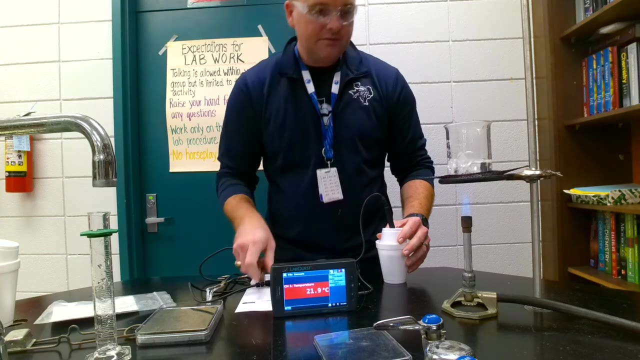 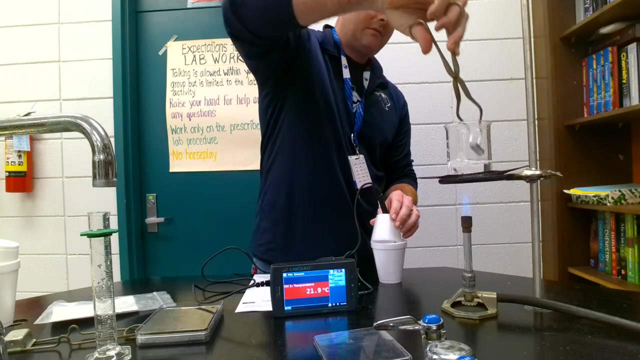 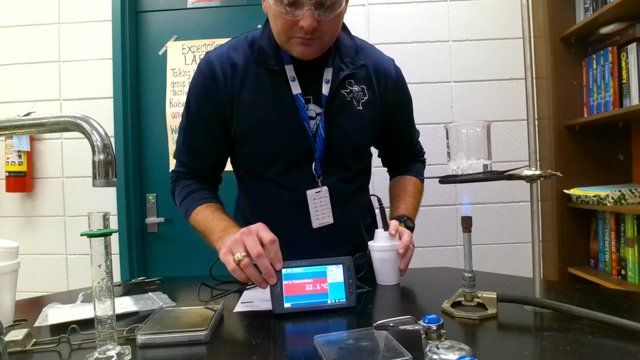 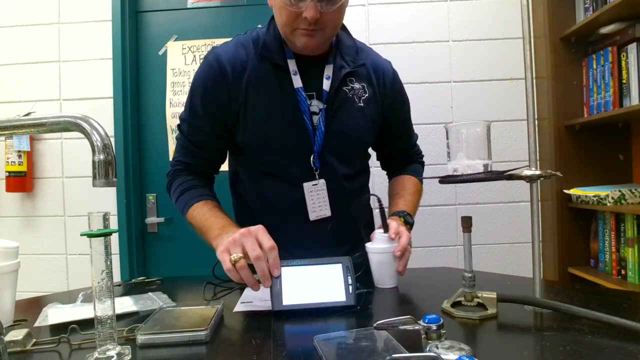 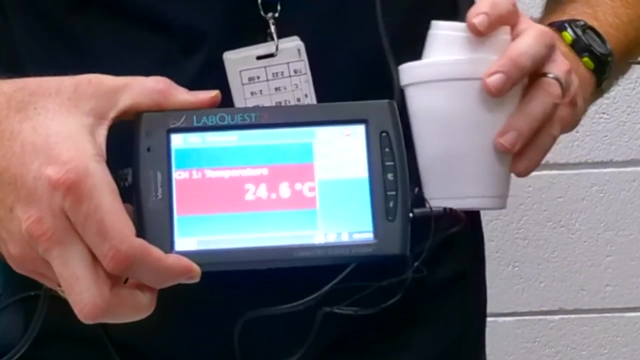 Okay, And that is going to be 21.9 degrees Celsius, And we're going to take this metal and we're going to take it out and put it in very quickly And the temperature should go up, Turn the gas off And we're going to go until we get to the highest temperature.